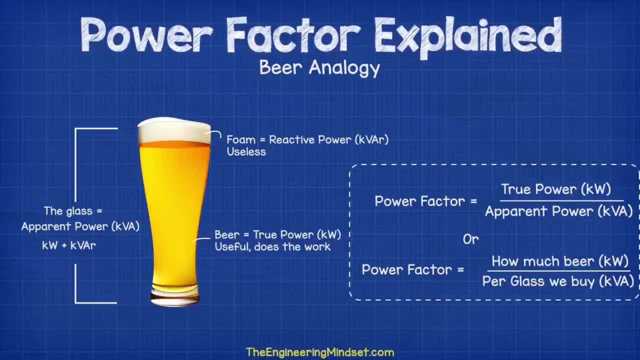 our KW divided by what we charge for in KVA, the kilovolt amps. So it's telling us how much value for money we're getting getting for the power we consume. If we briefly touch on electrical engineering- and I will keep this part brief- 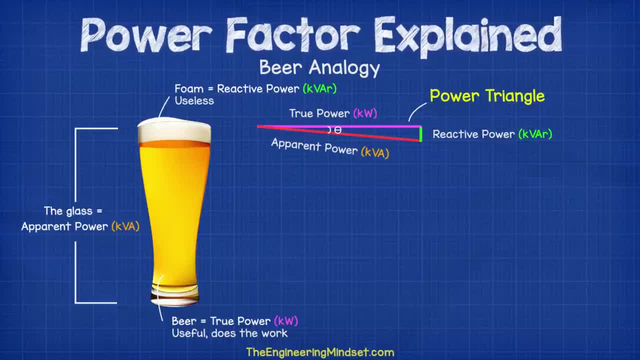 then we might see this expressed as a power triangle. In this case, I'll draw it as a leading power factor, as it's easier to visualize. The beer, or true power, is the adjacent line. Then we have the foam, which is the reactive power on the opposite. 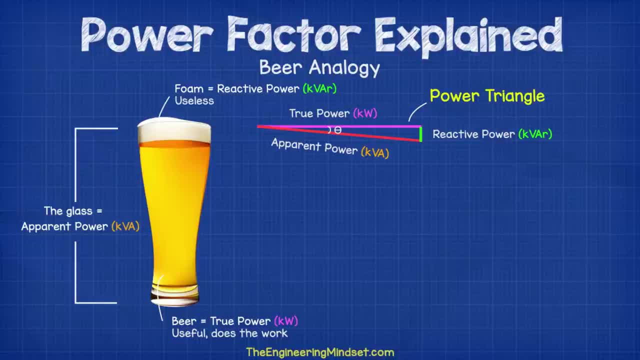 Then for the hypotenuse side, which is the longest side, we have the apparent power. This is at an angle from the true power. The angle is known as theta, You see, as the reactive power, or the foam, increases. 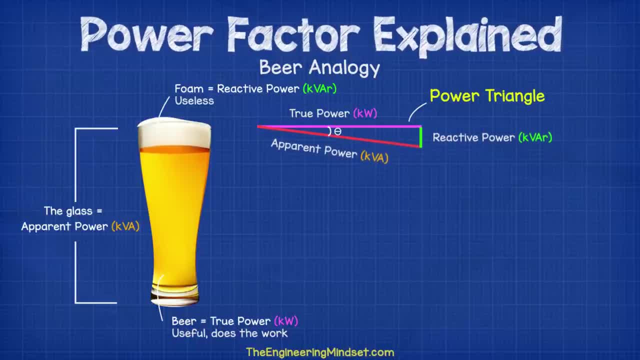 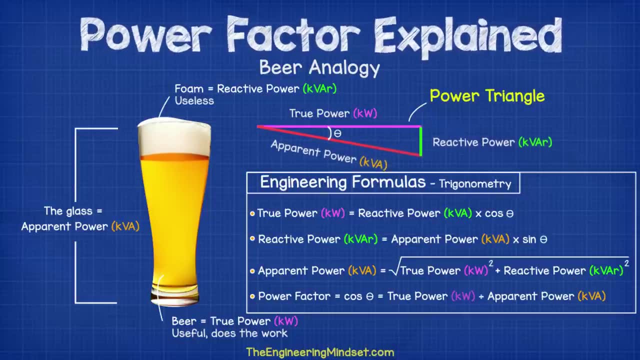 then so does the apparent power, or the kVA. We could then use trigonometry to calculate this triangle. I won't in this video, as I'm just covering the basics, so we'll just see the formulas you need, but we'll do some calculations and worked examples. 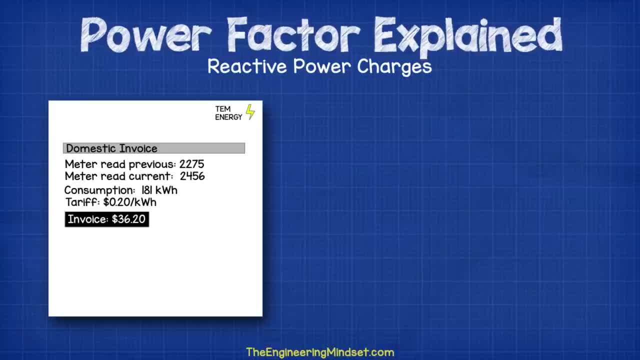 later in this video. If we look at a typical residential electricity bill, then we'll typically see just a fee for the amount of kilowatt hours used, because the power factor and the electricity consumption will be very low. See, electricity companies tend to not worry about this. 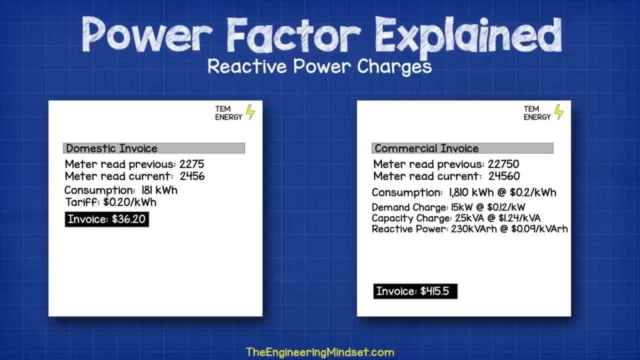 However, on commercial and industrial electricity invoices, especially buildings with smart or interval electricity meters, then we'll likely see charges and information for the amount of kilowatts, kilowatt hours, kilovolt amps and kilovolt amps- reactive used. 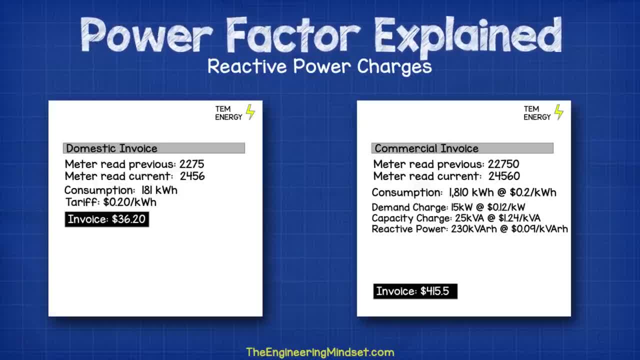 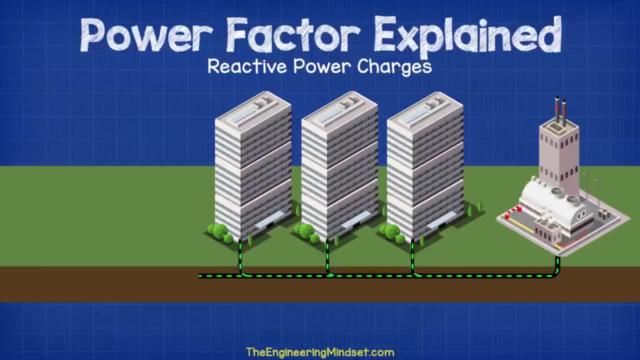 Large buildings in particular will often see reactive power charges in there, but this depends on the electricity supplier and the agreement they have with the consumer. The reason they charge a penalty for this is because when large consumers have bad power factors, they are increasing the current flow through the electricity. 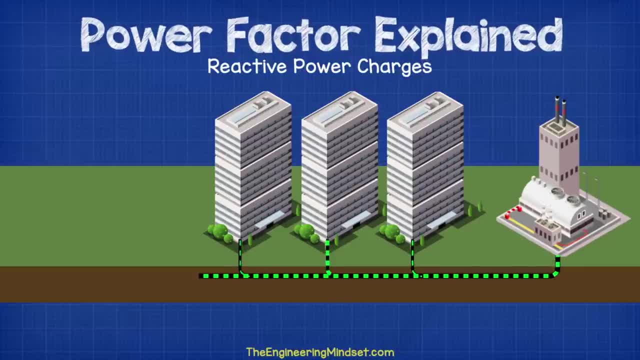 and the energy consumption. They're increasing the electricity network and causing voltage drops, which reduces the supplier's distribution capacity and has a knock-on effect for the other customers. Cables are rated to handle a certain amount of current flowing through them, So if a lot of large consumers connect with bad power factor, 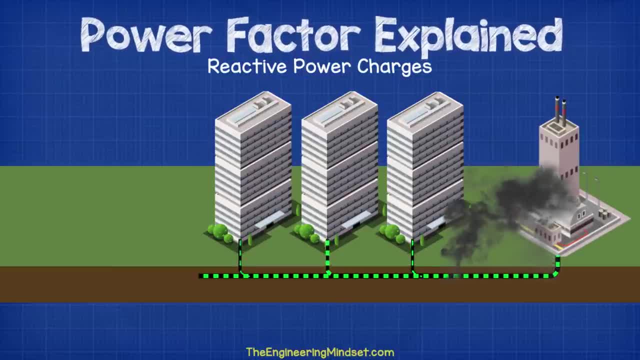 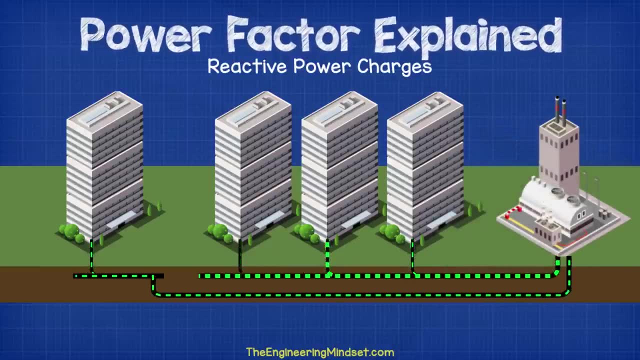 then the cables could overload, They could also struggle to meet the demand and the capacity agreements, and then no new customers will be able to connect until they either replace the cables or install additional cables. Reactive power charges occur when the power factor of a building 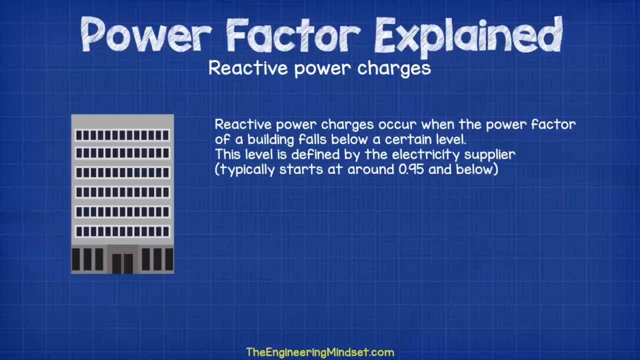 falls below a certain level. This level is defined by the electricity supplier, but it typically starts around 0.95 and below. A perfect power factor would be one. However, in reality, this is almost impossible to achieve. We'll come back to this part later in the video. 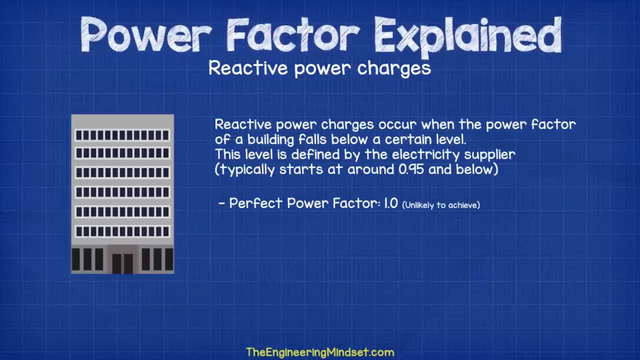 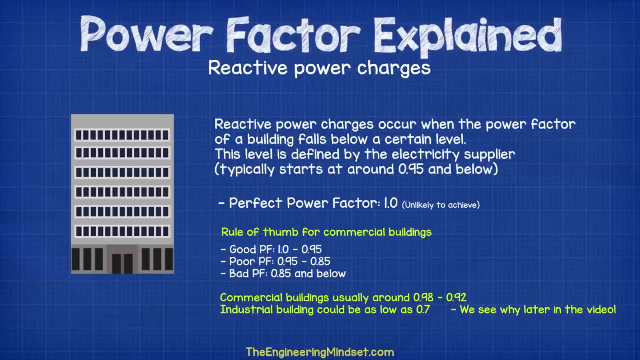 In large commercial buildings. the overall power factor is likely to sit in the following categories: Good power factor is generally between one and 0.95.. Poor power factor is anything from 0.95 to 0.95.. Poor power factor is anything from 0.95 to 0.95. 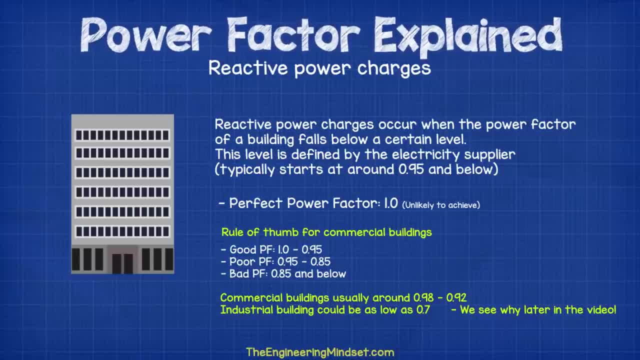 Bad power factor is anything from 0.95 to 0.95.. Bad power factor is anything below 0.85.. Commercial office buildings are usually somewhere between 0.98 and 0.92.. Industrial buildings could be as low as 0.7.. 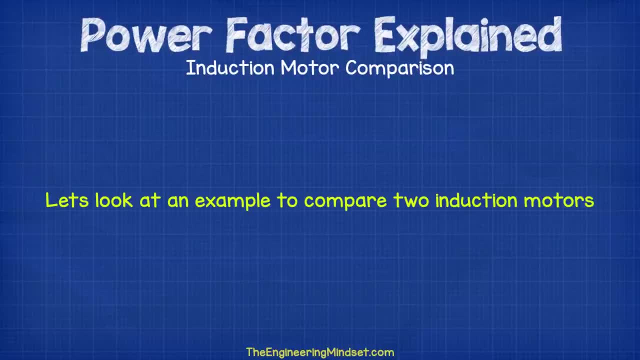 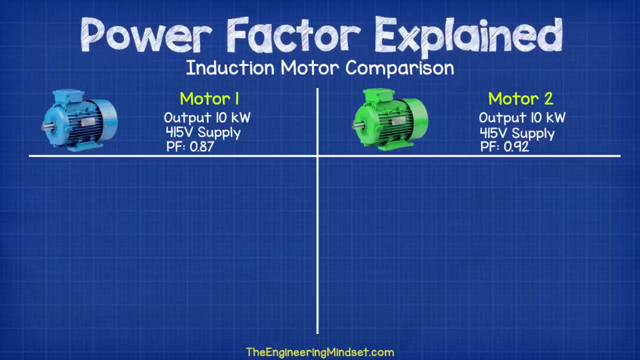 We'll look at what causes this shortly. Let's first have a look at an example. If we compare two induction motors that both have an output of 10 kilowatts and are connected to a three-phase 415, 50 hertz supply. 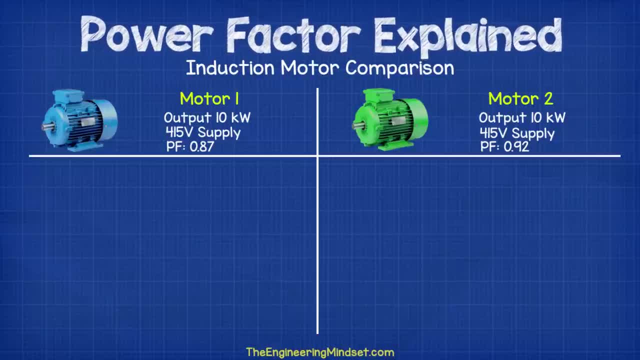 one has a power factor of 0.95,, one has a power factor of 0.87, and the other with a power factor of 0.92.. Both motors will deliver 10 kilowatts of work, but the first motor has a lower power factor. 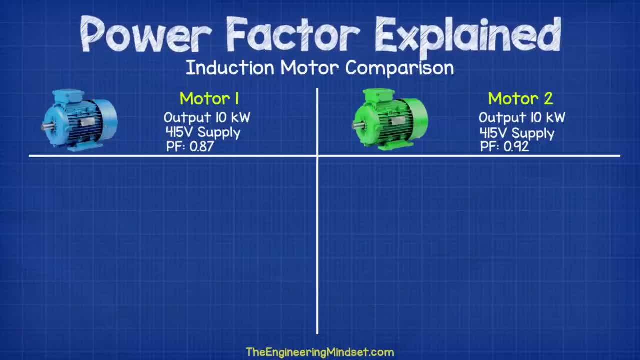 compared to the second one, meaning we're not getting as much value for money. The first motor will need to draw 11.5 kVA from the electricity grid to provide the 10 kilowatts of power. The second motor will need to draw just 10.9 kVA. 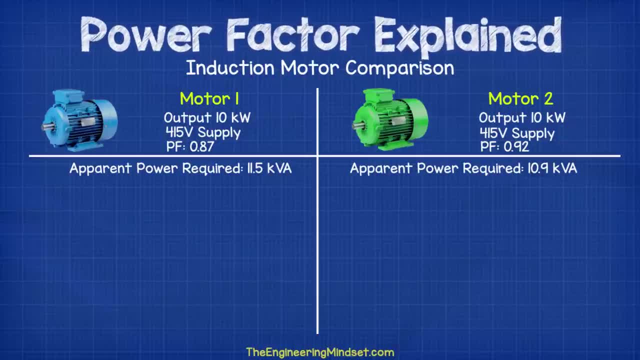 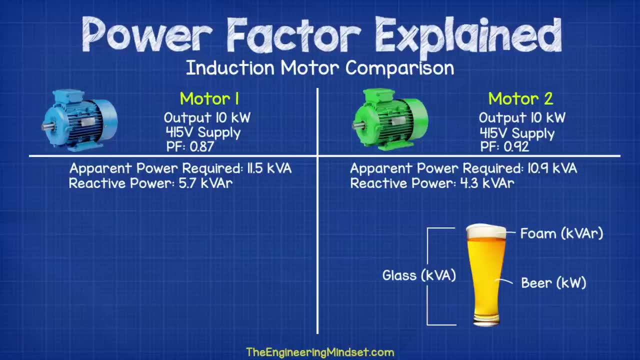 from the electricity grid to provide the same 10 kilowatts of power. This means the first motor has 5.7 kVars and the second motor has just 4.3 kVars. Remember, our kilowatts is the beer and that's the useful stuff. 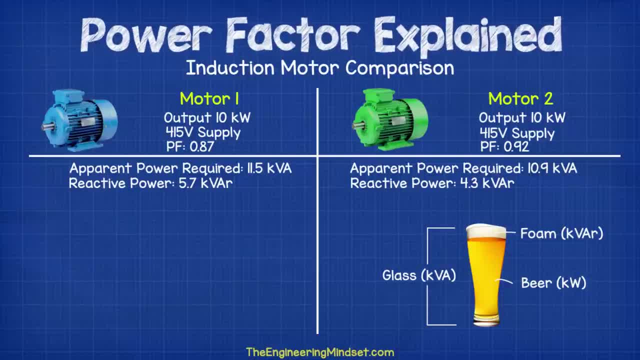 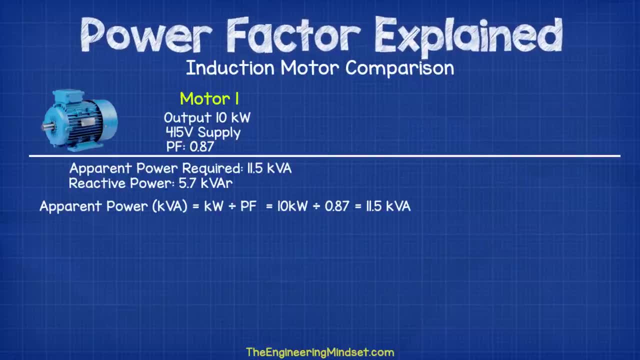 The kVars are the foam, that's the not-so-useful stuff. The kVA is what we're going to pay for, and that's the kilowatts and the kVR combined. How did I calculate that For kVA I used kilowatts divided by power factor. 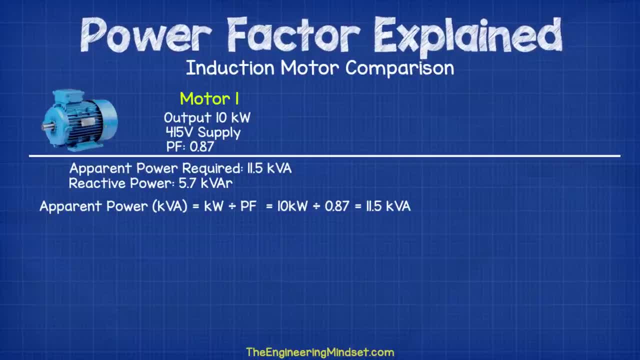 so 10 divided by 0.87 to get 11.5 kVA. For kVA I used the square root of kVA squared subtract kilowatts squared, So the square root of 11.5 kVA squared minus 10 kilowatts squared. 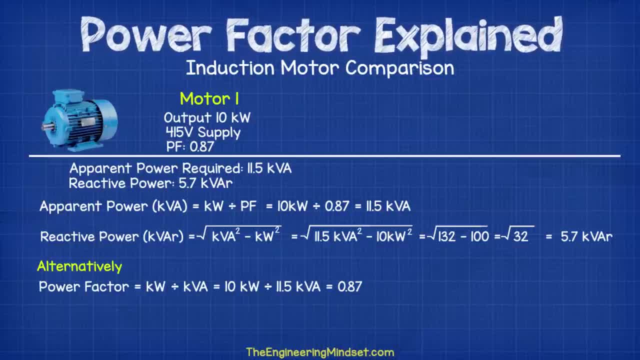 We could have also found the power factor from the kilowatt and the kVA using 10 kilowatt divided by 11.5 kVA. We could have found the kilowatts from the power factor and the kVA using 0.87 divided by 11.5 kVA to get 10.. 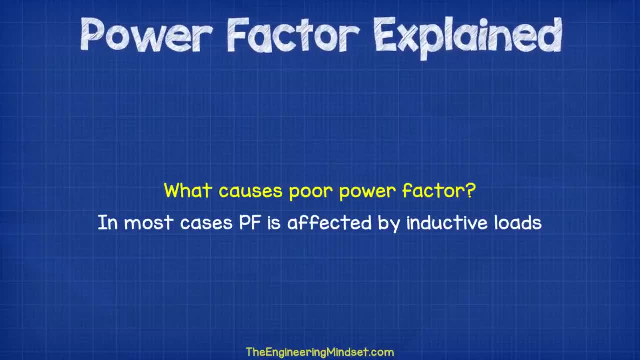 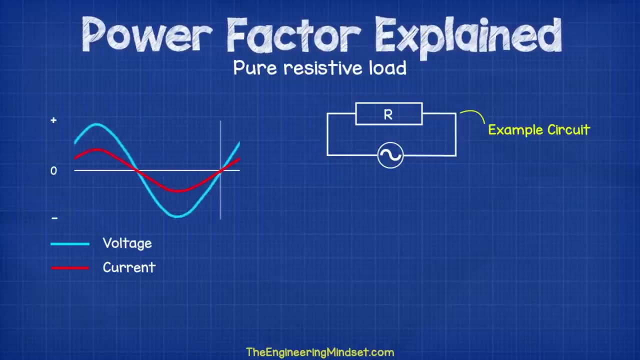 So what causes poor power factor? In most cases, the power factor is affected by inductive loads. If we have a purely resistive load, such as an electrical resistive heater, then the voltage and the current waveforms would be in sync or very close. 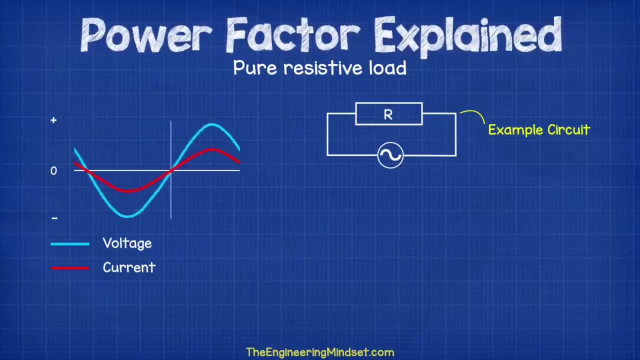 They would both pass through their maximum and minimum point and then pass through the zero axis at the same time. The power factor in this case is one which is perfect. If we drew a phasor diagram, then the voltage and current would be parallel. 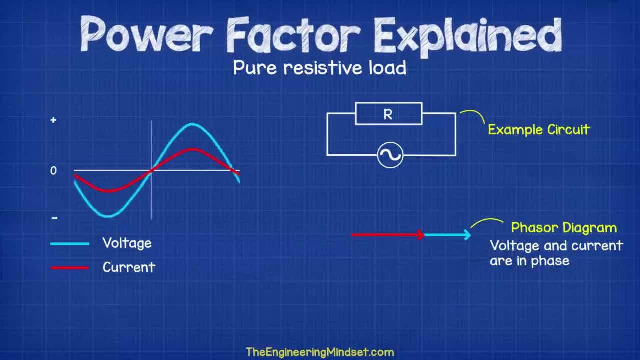 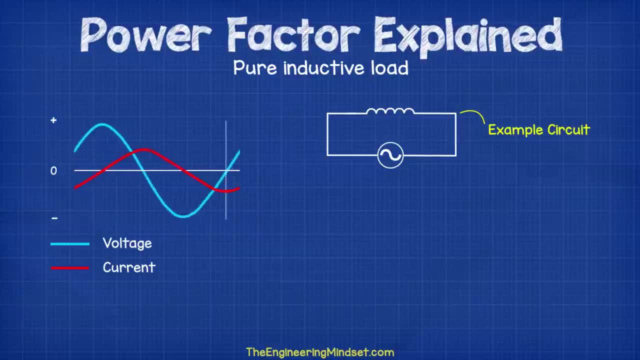 So all the energy drawn from the electricity supply goes into doing work, in this case creating heat. But if we took an inductive load as an induction motor, then the coil's magnetic field holds back the current and results in a phase shift where the voltage 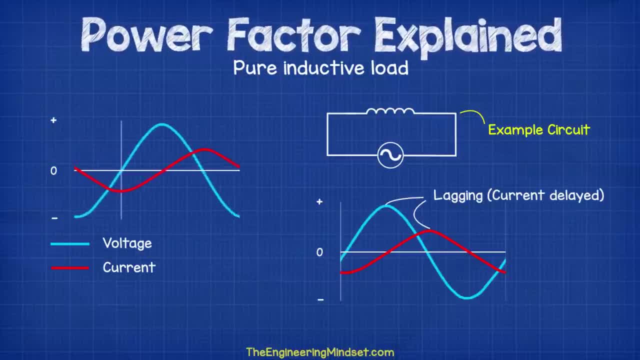 and the current waveforms fall out of sync with each other, so the current passes through the zero point after the voltage. This is referred to as a lagging power factor. Earlier in the video I said the foam or the kVA is useless. 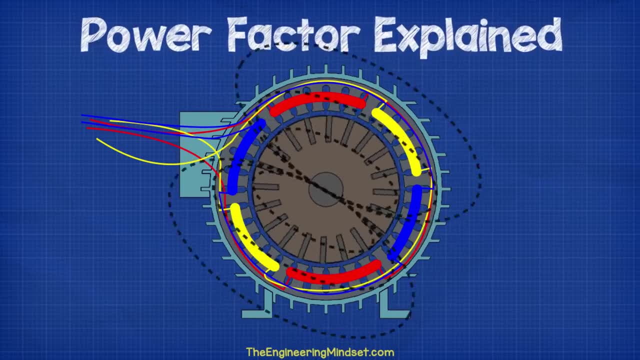 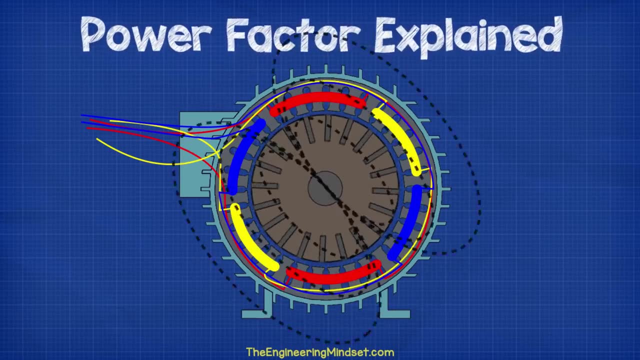 That's not exactly true. We actually need some reactive power to create and maintain the magnetic field which rotates the motor. The reactive power is wasted in the sense that we get no work from it, but we still have to pay for it, although we do need it to be able to do the work. 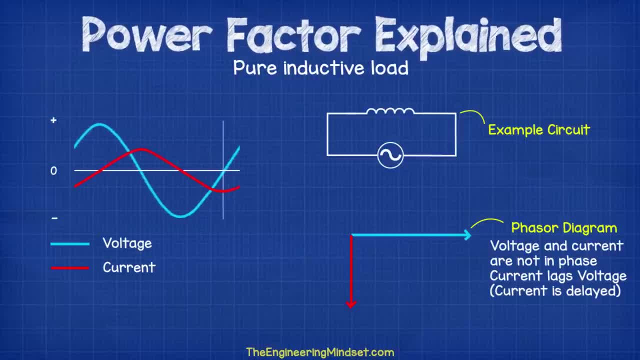 in the first place. If we drew a phasor diagram for a purely inductive load, then the current would be at an angle below the voltage line, meaning not all the electricity consumed is doing work. If we took a purely capacitive load. 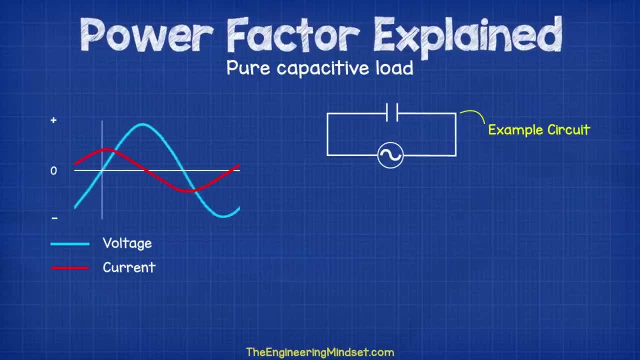 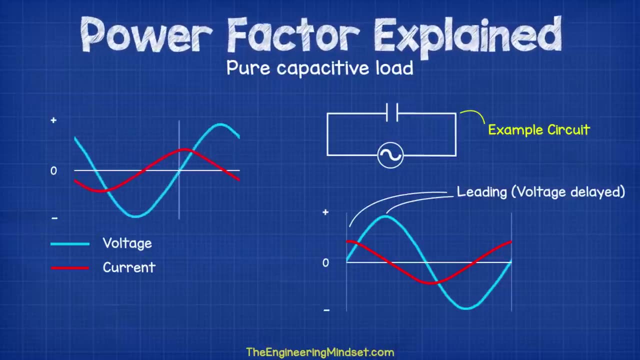 then the opposite happens to the inductive load. The voltage and current are out of phase, except this time the voltage is held back. This causes leading power factor Again. this will mean that not all the electricity being used is being used to do work. 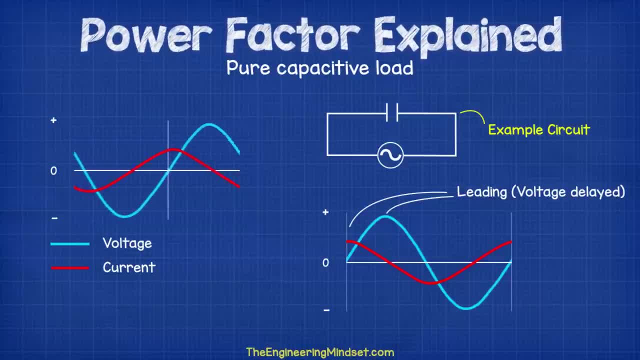 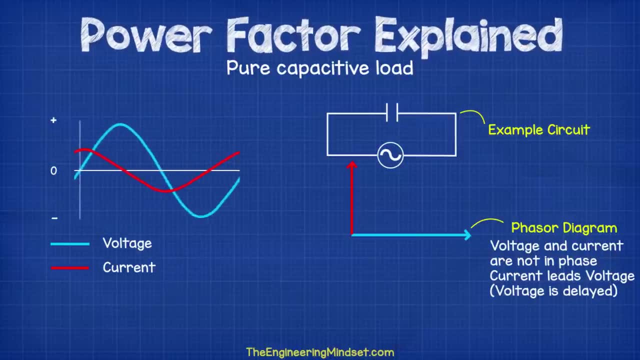 but we still have to pay for it regardless. If we drew a phasor diagram for a purely capacitive load, then the current line would be at an angle above the voltage line as it's leading, Correcting poor power factor. What can we do to correct poor power factor? 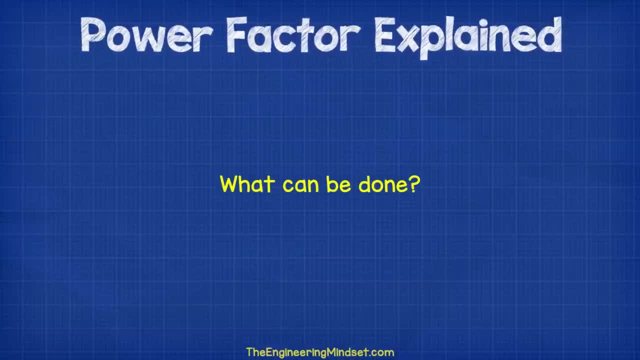 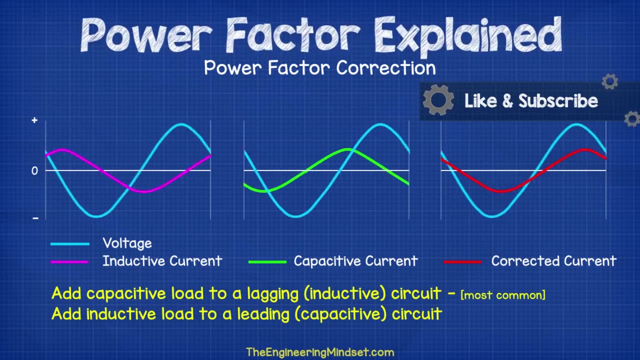 and reactive power charges. In most cases we come across lagging power factor caused by inductive loads. To correct poor power factor, we can add capacitors or inductors to the circuit, which will realign the current back into phase and bring the power factor closer to one. 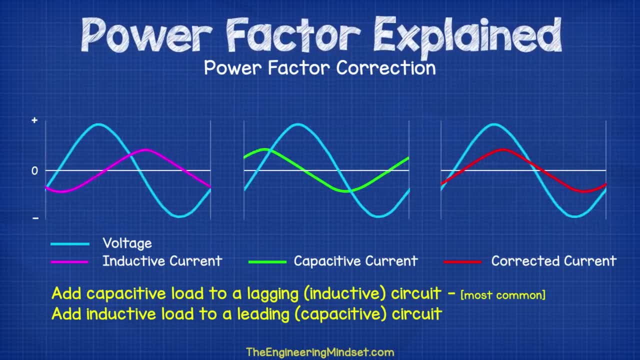 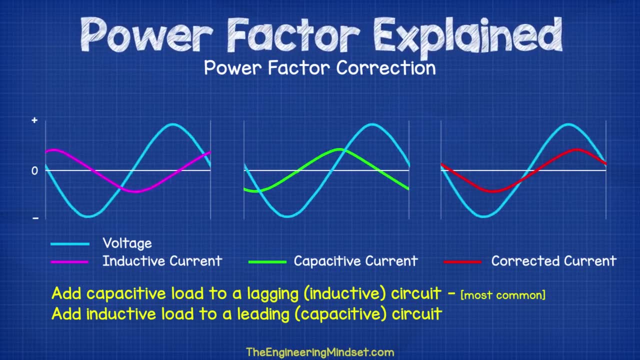 If we have a lagging power factor caused by high inductive loads in the circuit, then we add capacitors. If we have a leading power factor caused by high capacitive loads, then we add an inductive load to the circuit. These need to be calculated. 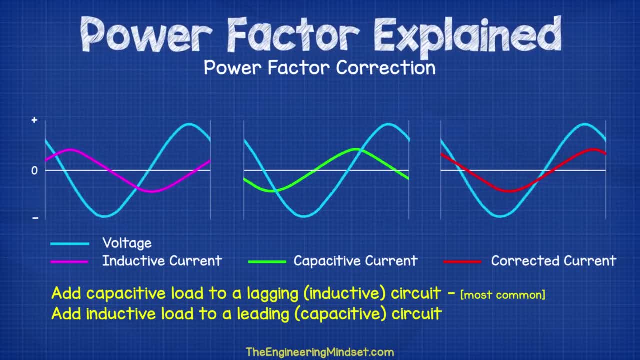 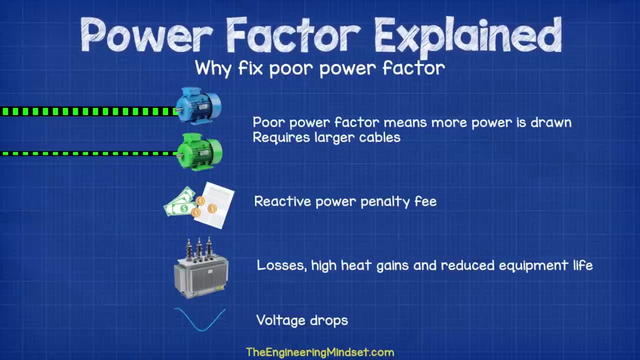 and we'll see some example calculations of this at the end of the video. So why should we fix poor power factor? Poor power factor means you need to draw more power from the electricity network to do the same amount of work. Therefore, the cables need to be larger. 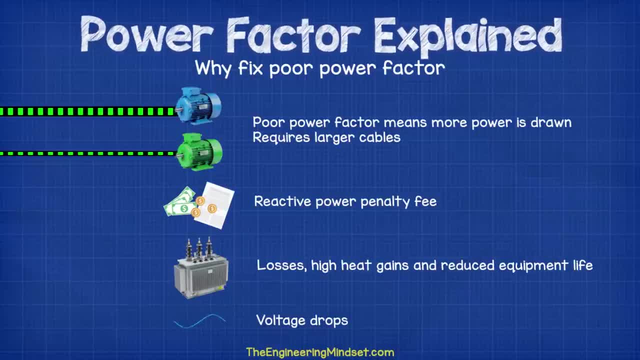 so the installation is going to cost more money. If the power factor becomes too low, then the electricity supplier might charge you a penalty fee or a reactive power charge. Poor power factor can cause losses in equipment like transformers and leads to high heat gains. 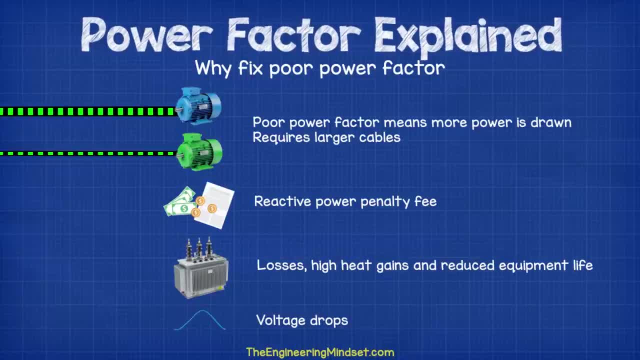 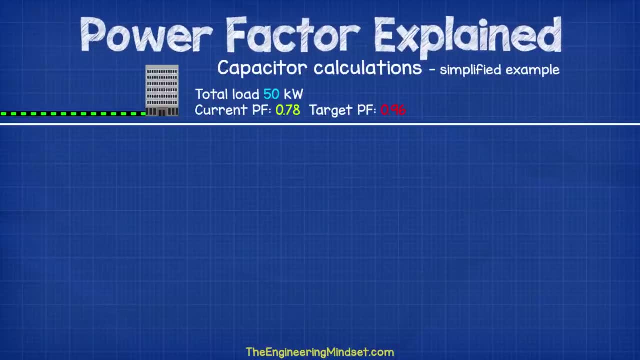 It can lead to voltage drops and can even reduce the life expectancy of equipment in extreme scenarios. Capacitor calculations for power factor correction. Let's look at a simplified example of calculating the size of a capacitor to improve the power factor of a load. The building has a three-phase power supply. 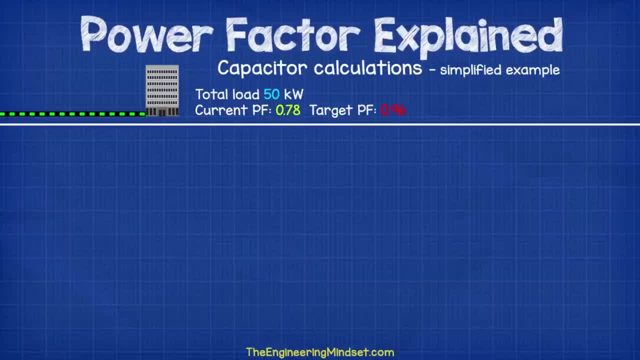 and has a total load of 50 kilowatts of work. It also has a power factor of 0.78, but we want it to be 0.96 to avoid penalty charges. Currently, the building has a total apparent power or KVA value of 64.1 KVA. 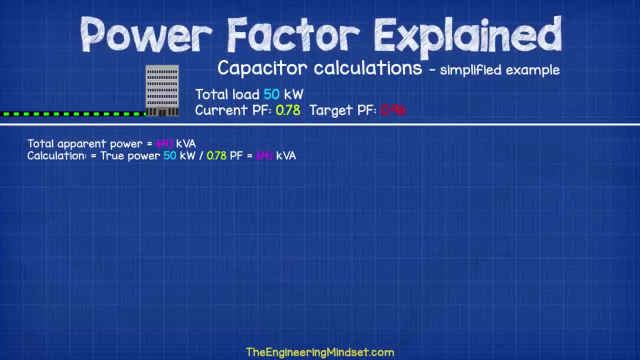 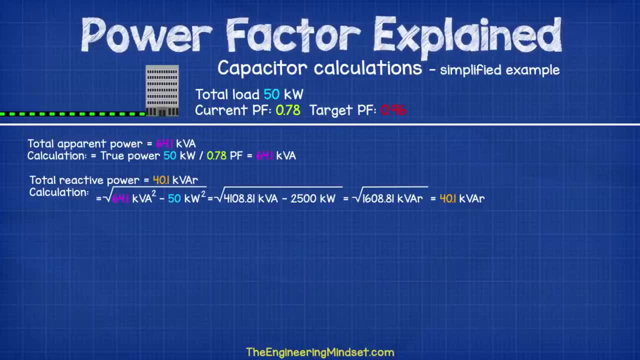 And we find that by just dividing the kilowatts- 50 kilowatts- by the power factor of 0.78, it also has a reactive power of 40.1 KVA. We find that by taking the square root of the KVA squared.